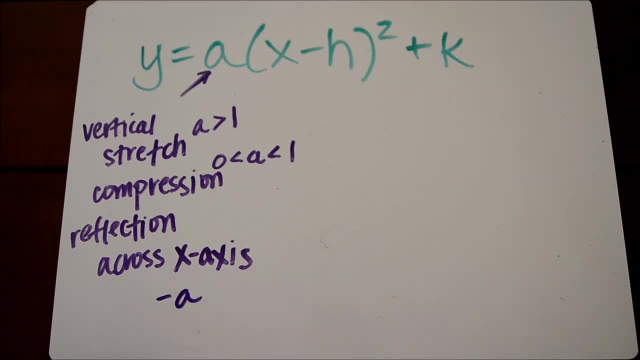 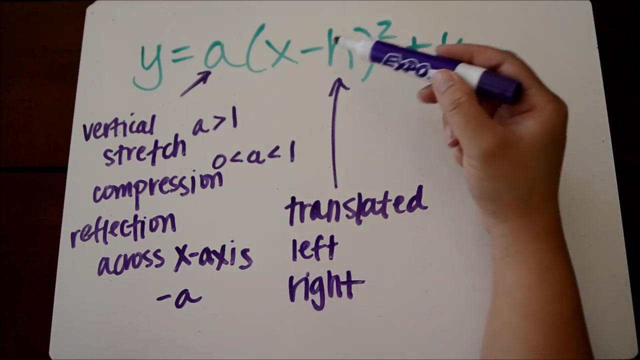 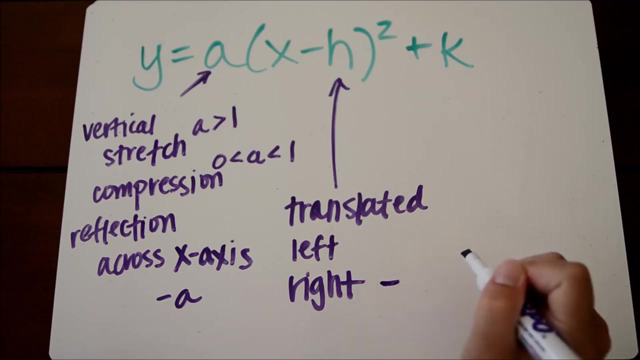 graph looks wide And if the a value is negative we have a reflection across the x-axis, which means our graph opens downward. The h value tells us if our graph was translated left or right. So you'll notice that vertex form has a minus sign in here. so this is a little tricky If that minus. 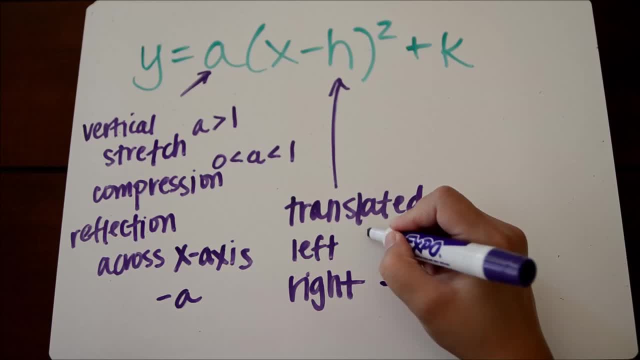 sign is still there, it actually means our graph moved to the right. If you see a plus sign there, it means our graph translated to the left, And I'll talk about that a little bit more on our next slide, because that's a little counterintuitive. Our k value tells: 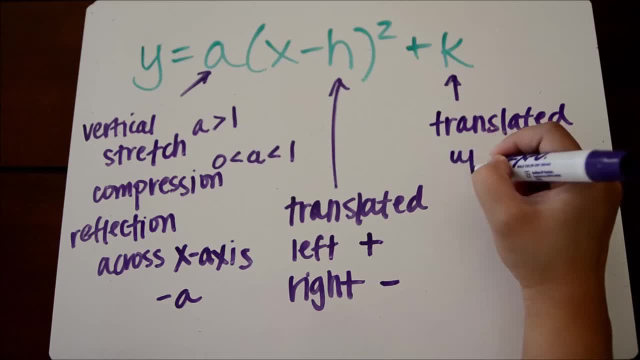 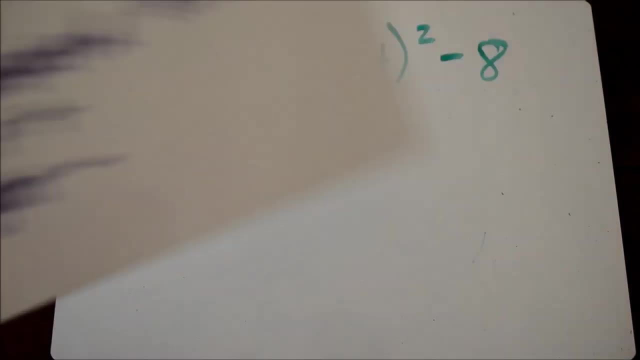 us our translation up or down. but this does what you think it should do. If it's plus k, our graph translates up. If it's minus k, our graph translates down. All right, let's take a look at our first example. So here we have y equals 3 times. 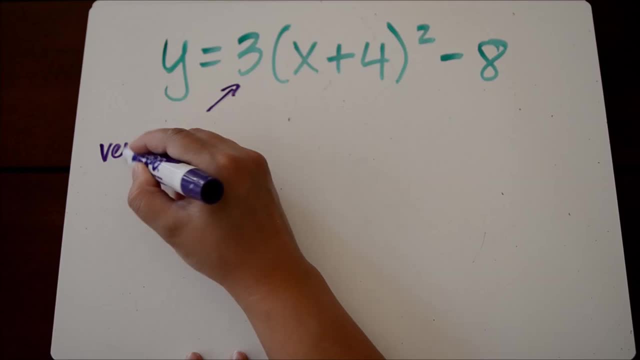 the quantity of x plus 4 squared minus 8.. The 3, our a value, tells us we have a vertical stretch. So we're looking at a rotational strip of a block. in here, t db equals y times a derivative of x plus 4 squared minus 8.. Our a value tells us we have a vertical stretch. 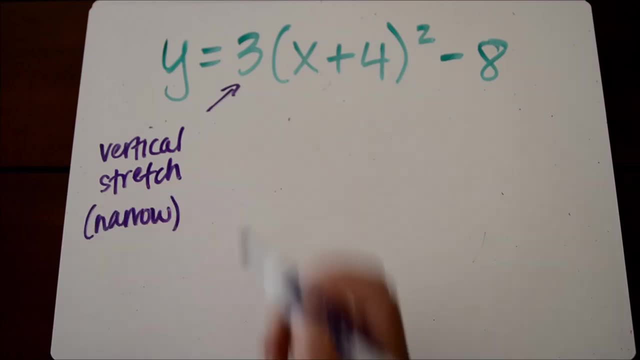 The vertical line comes痛 matters. And if we take the three Meskin line, which is inJin premiers, because that's a number that's bigger than one, That means our graph is going to look a little narrow. Our h value here, remember, 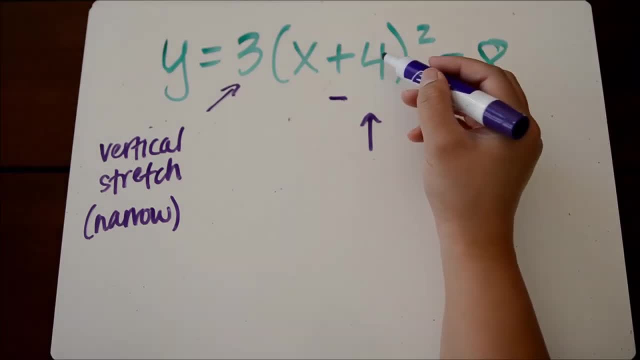 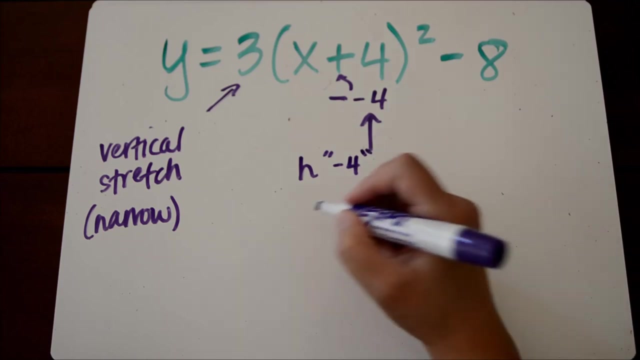 we had a minus sign in vertex form, so this is actually minus a negative four. That's how it becomes plus four. So since our h value is actually a negative four, what that means is our graph went to the left four units, And I know that seems very counterintuitive. 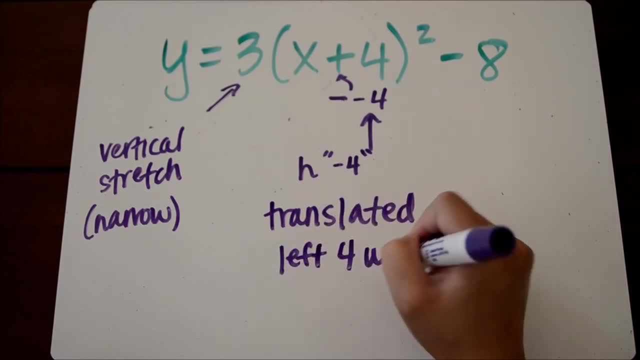 because it says plus four. If you need to think about it as doing the opposite, then you can think about it that way, But there's a reason and it's because it's minus a negative. Okay, so let's take a look at our k value. 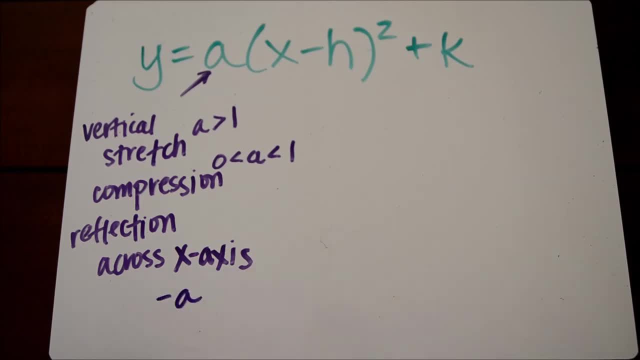 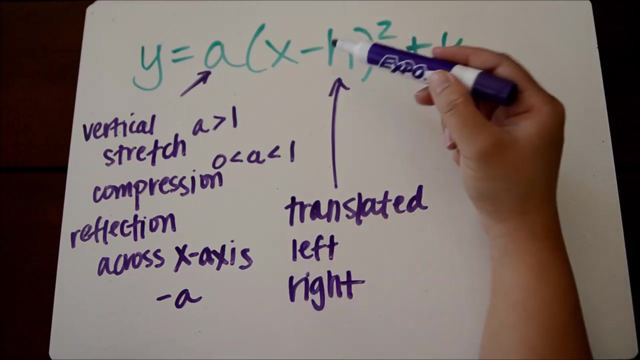 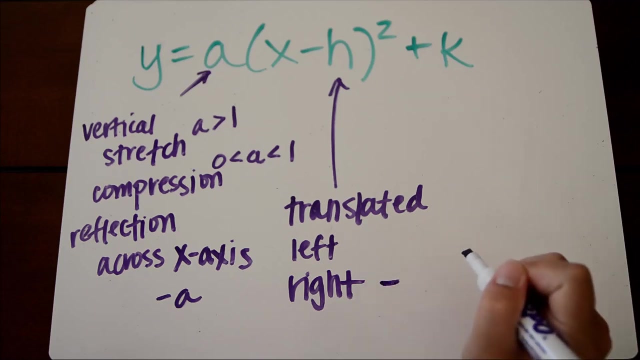 looks wide And if the a value is negative we have a reflection across the x axis, which means our graph opens downward. The h value tells us if our graph was translated left or right. So you'll notice that vertex form has a minus sign in here. So this is a little tricky If that minus. 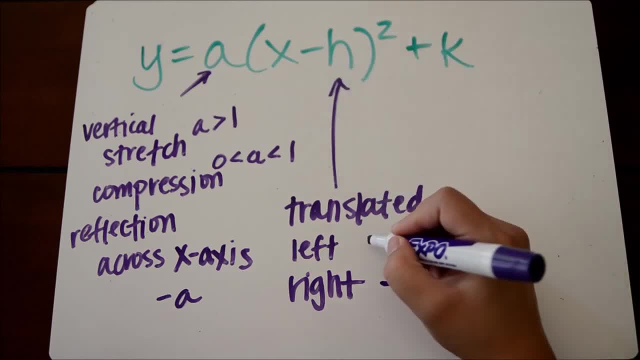 sign is still there, it actually means our graph moved to the right. If you see a plus sign there, it means our graph translated to the left, And I'll talk about that a little bit more on our next slide, because that's a little counterintuitive. Our k value tells: 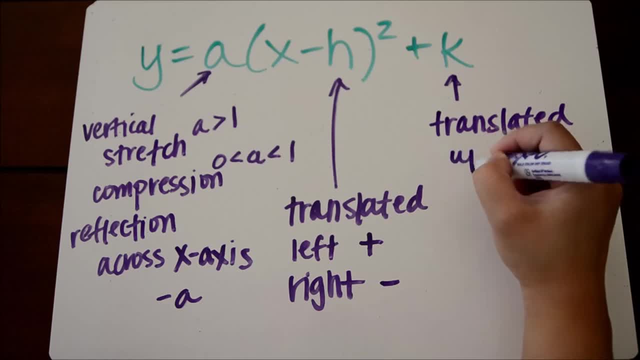 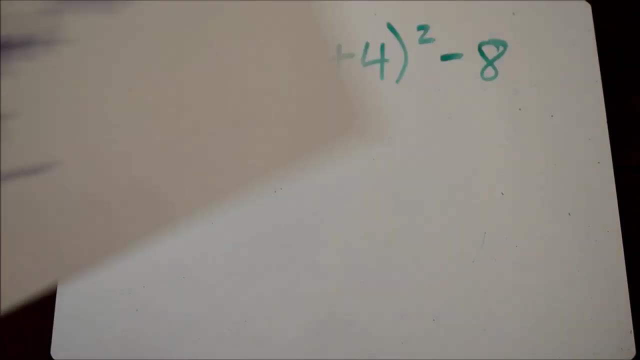 tells us our translation up or down. But this does what you think it should do: If it's plus k, our graph translates up. If it's minus k, our graph translates down. All right, let's take a look at our first example. So here we have: y equals 3 times the quantity of x plus 4 squared. 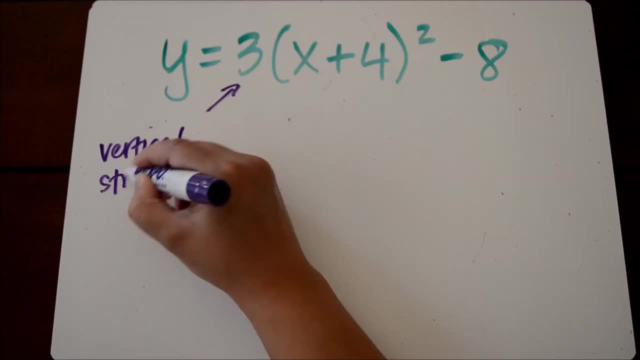 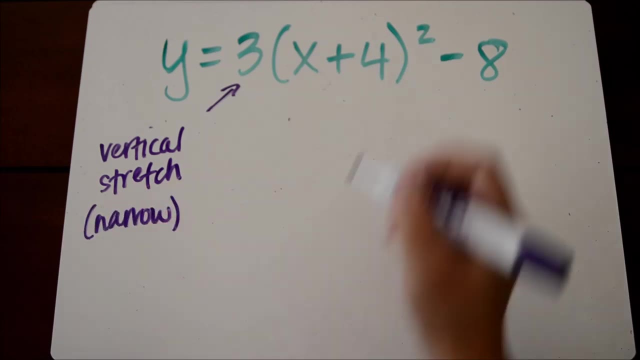 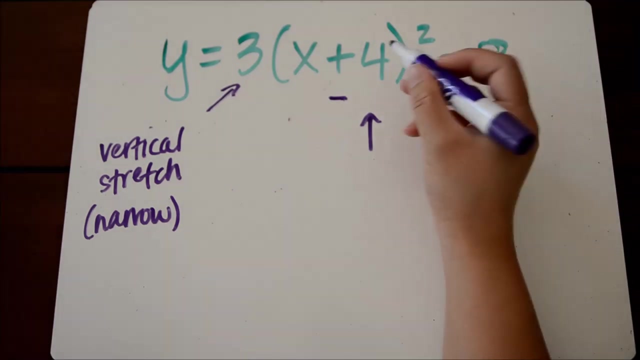 minus 8.. This 3, our a value tells us we have a vertical stretch, because that's a number that's bigger than 1.. That means our graph is going to look a little narrow. Our h value here- remember we had a minus sign in vertex form- so this is actually minus a negative 4.. That's how it becomes. 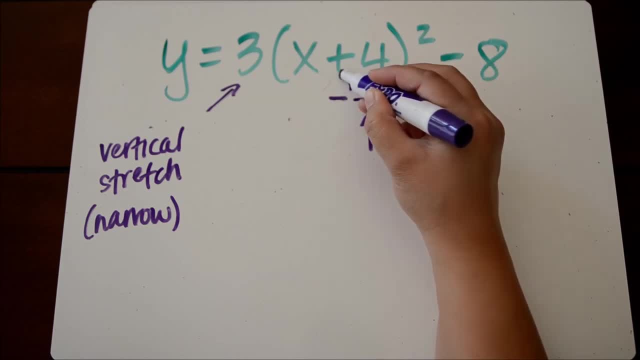 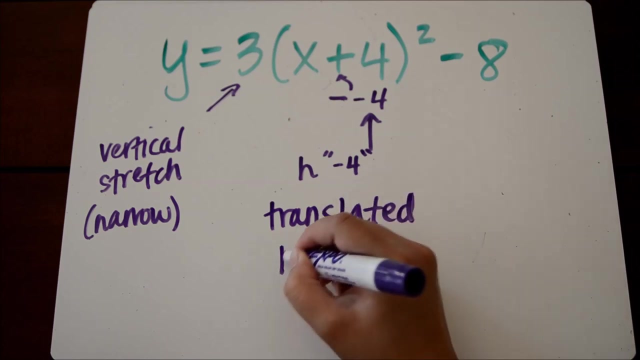 plus 4.. So since our h value is actually a negative 4, what that means is our graph went to the left four units, And I know that seems very counterintuitive because it says plus four, If you need to think about it as doing the opposite. 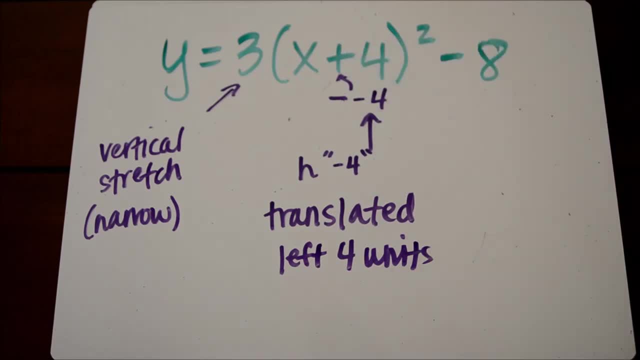 then you can think about it that way, But there's a reason and it's because it's minus a negative. Okay, so let's take a look at our k value. It's a negative eight And our k value does what we think it should do.